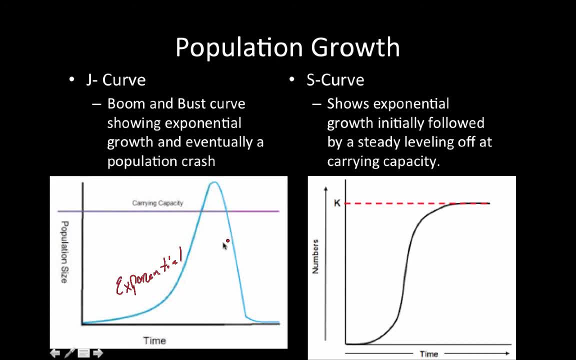 all the way up, and then usually it leads to population crash. so this is another one we can call a boom and a bust. Alright, so we could call it that way too, but this is our J for sure, and it kind of looks like a J. right, we'll see that J. 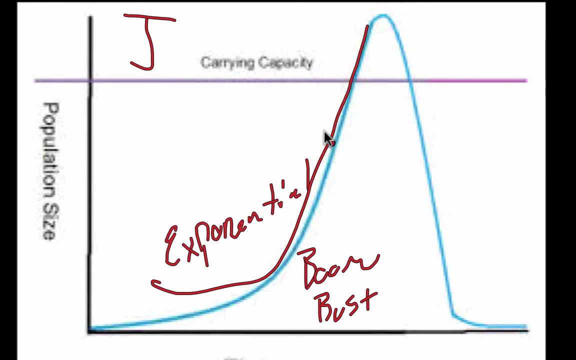 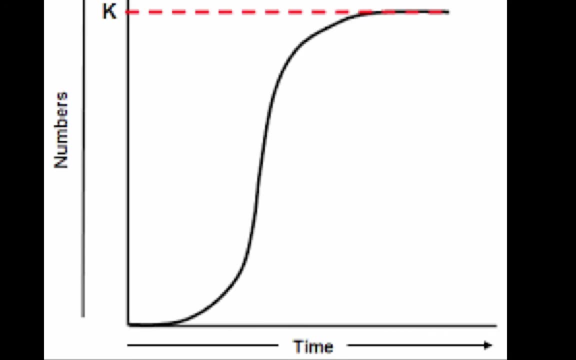 right there. What does this represent? It represents an organism's population exceeding carry capacity, running out of resources and then dying off. It doesn't always die off all the way. A lot of times it just has to dip back below carrying capacity and can level out again. If it does level out again, then what we? 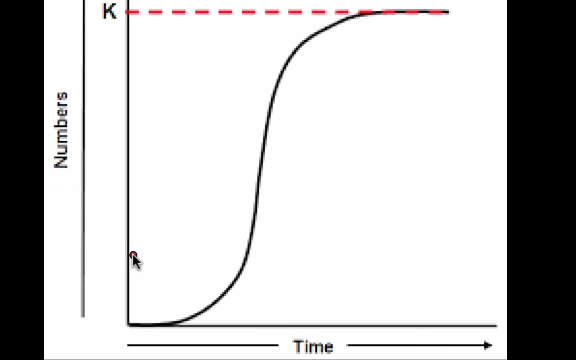 see, is really an S-curve start to unfold. Here we see our S-curve. So what do we have? We have exponential growth all the way up to here. It's exactly the same as a J-curve. Here we see this. 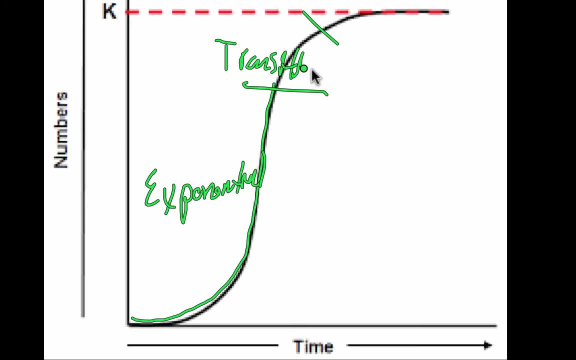 little transition. Here we see a plateau phase, so it levels off. So we have kind of a one, two, three. What happens? why does it level off? Well, it levels off because of this same reason. up here The population usually exceeds carrying capacity. It doesn't level off perfectly. 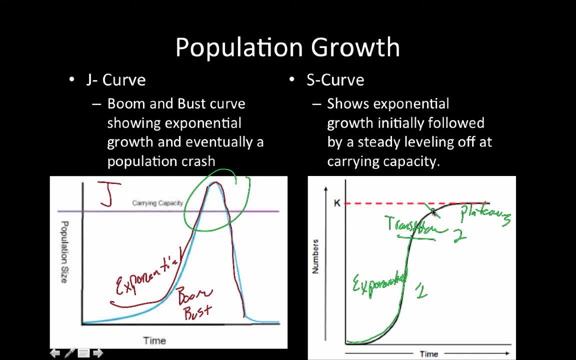 like this. Usually what it looks like is on the previous slide you saw one too- but you'll see the population kind of transition and then exceed and then some start to die off. Then it dips below and we see this Now: this red line is still carrying capacity, but we see population kind of go above. 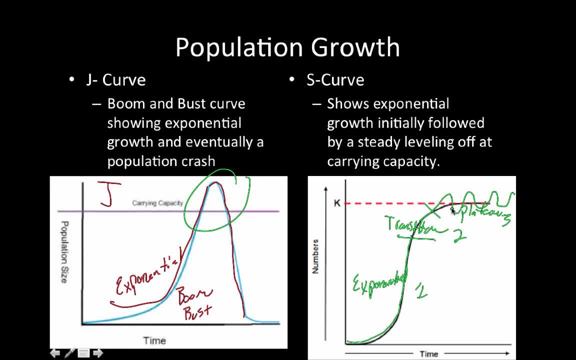 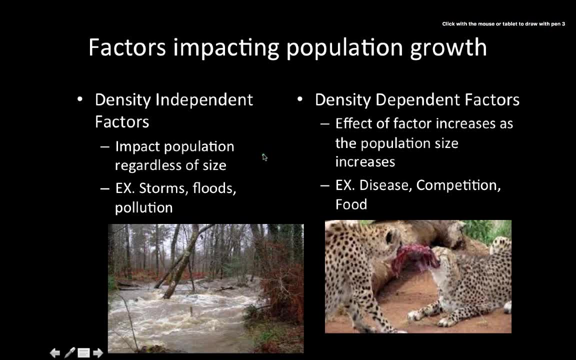 and below, depending on the resources that are available and the struggle for survival. So what are some key factors for impacting population growth? We have density independent factors and density dependent factors. The easiest way to keep them separate, to understand them better, is to think about. 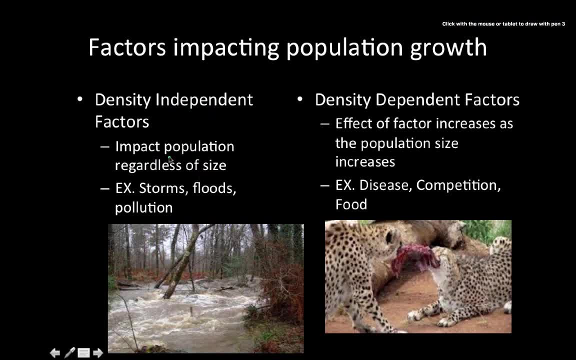 if it's independent, it's doing it by itself, regardless of population size, So it's going to impact animals in exactly the same way, no matter how packed together they are or not. Perfect examples are storms, floods, fires, pollution- Those things are going to harm the same number of animals. 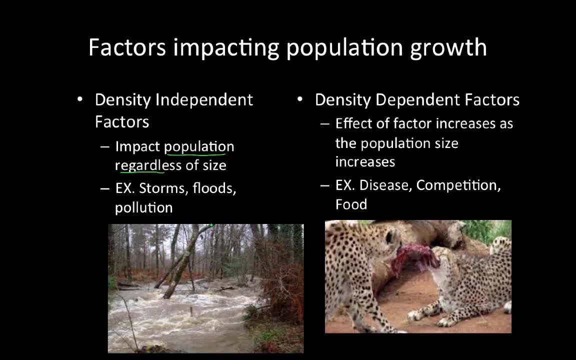 in an ecosystem, no matter how packed together the population is, It's impact is going to be the same. So think about it this way: A storm that goes into a forest is not going to be stronger if there's a thousand birds or one bird Right. The storm is just going to be the storm and it's going to. 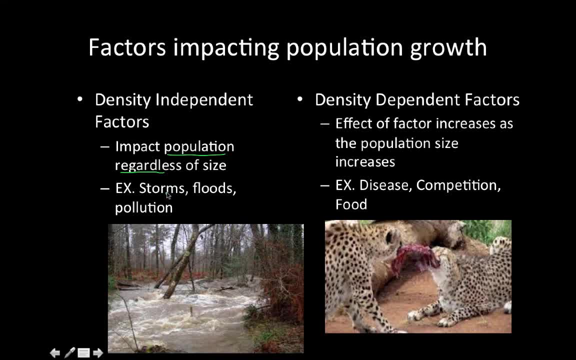 knock down just as many trees as it would regardless of how many animals were there. Density dependent factors actually increase based on the density of those organisms. So the factor is going to increase based on the population size. Something like disease competition for food. all those things are going to be. 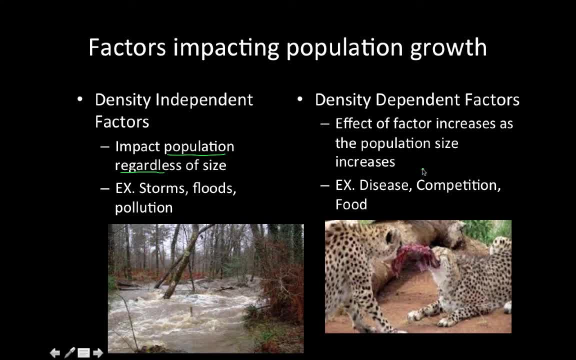 density dependent Disease in particular is a big one about it. if there's people packed closely together in a room, is a cold or a flu going to spread faster- absolutely so. the impact of that colder flu is going to be higher if the population is higher. 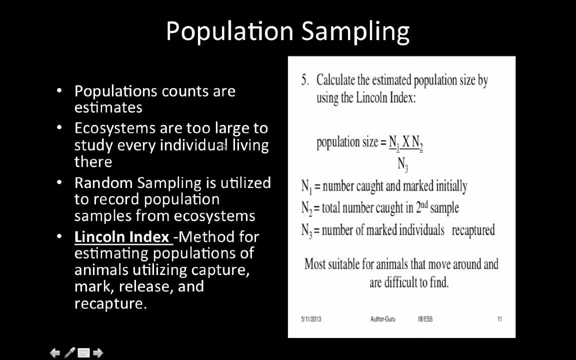 population sampling is something we'll we'll discuss in class. so there's two things we can do. we basically estimate the population of organisms in the ecosystem. we look at animals one way and plants another way. the keys takeaways for population sampling are this and this is: 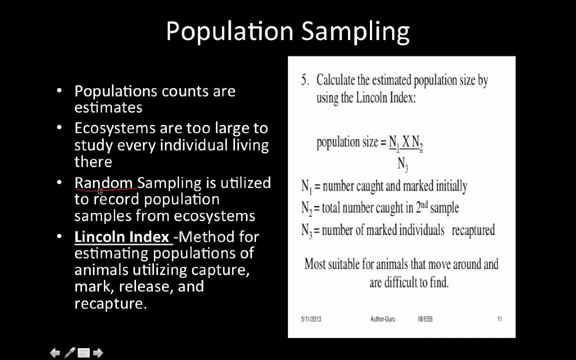 talking about animals, it has to be random and same with plants. random sampling is important. there can't be biased. we don't want. we want to eliminate bias. we want to utilize population samples from ecosystems. why do we sample? why don't we just go out and count every animal? okay, maybe with deer. 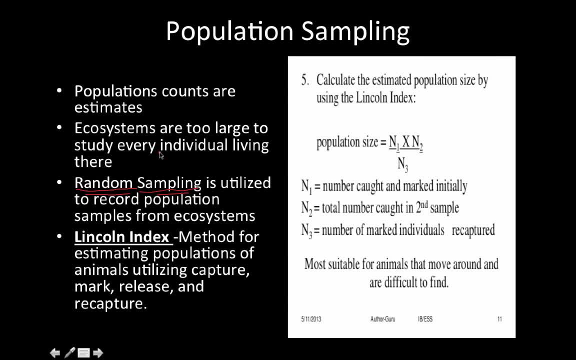 that's something we could do. that'd be really hard. think about all the ants in an ant hill. there's five hundred animals that live in an ant hill and then we get to the first one and we do that: thousand ants in an ant hill. how do you count them all? How do you get to them Especially? 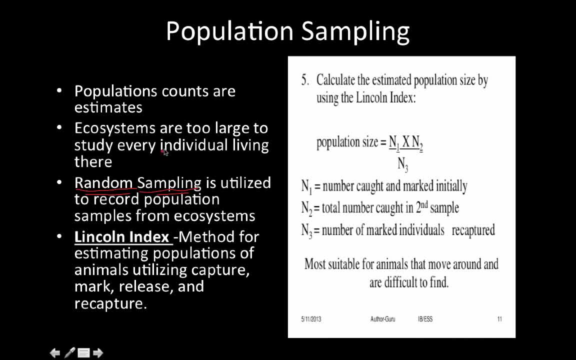 without disturbing their entire environment. So we have to remember that estimates are as good as we can do in population sampling. Ecosystems are just too large to study every individual. So because they're too large, we can't count them all. They're going to be an estimate. 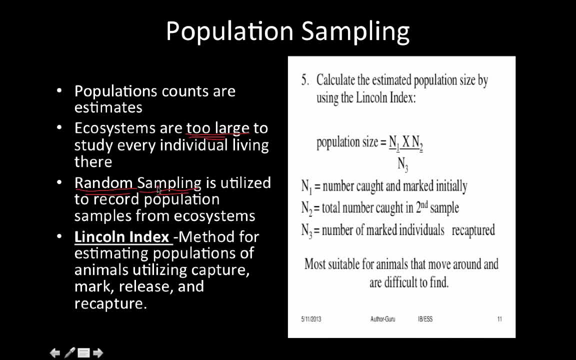 If we're going to estimate something accurately, it has to be done randomly, So we take our bias away. The Lincoln Index is a way to do that. It's also referred to as capture mark release recapture. See that down here. And the formula for that is right here: N1 times N2 divided by N3.. 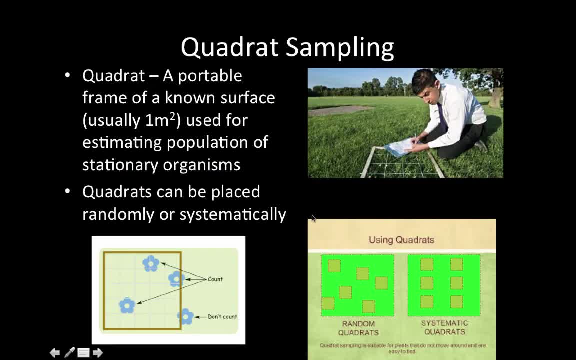 And we'll work on that in class that is showing examples here. Estimating populations of plants is done differently For animals. we do that: capture, mark, release, recapture. The index is a way to do that And we'll work on that in class that is showing examples here. 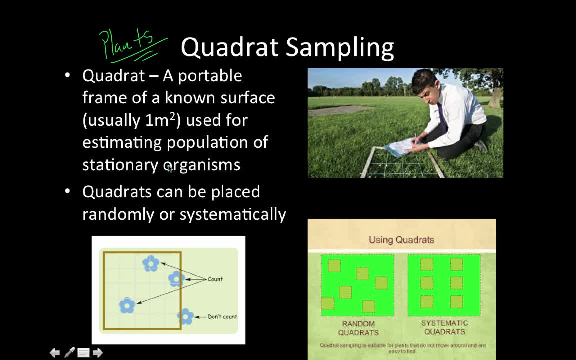 The issue with plants is you don't really capture plants because they're stationary, So that doesn't make a whole lot of sense. What we can do is sample plants in their natural environment, still randomly, using this tool called a quadrat. It's just basically a square. 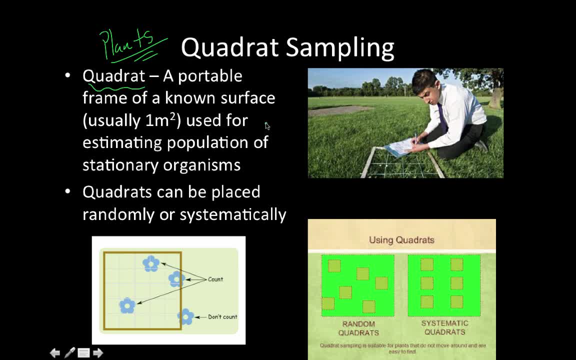 portable frame, usually one meter In class. ours are going to be a half a meter or 0.5 meters squared Quadrat is what we'll use. The quadrat can be placed randomly or systematically, No matter what we're sampling. 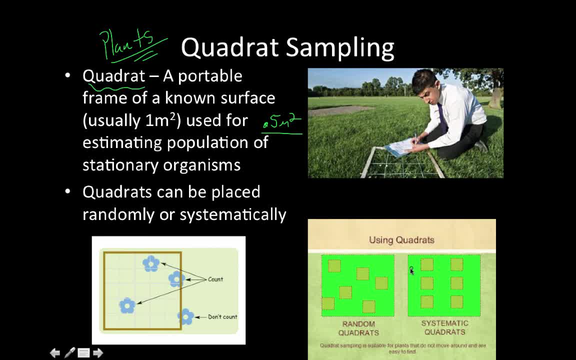 We're sampling a random part of the ecosystem, Even if it's systematic. that just means laying them in rows. So maybe this is like we're looking at it and saying this is going to be one meter here, one meter here and two meters here difference, All right. 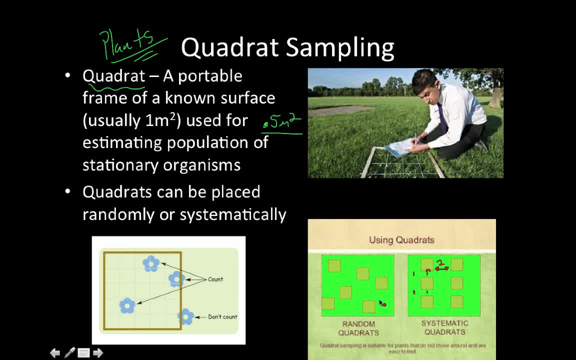 That's all they're saying. Where random is just kind of randomly placed, It's usually a table of numbers, a random table of numbers that allows us to place it here on a grid system. That's the best way, Or they can just be thrown randomly. 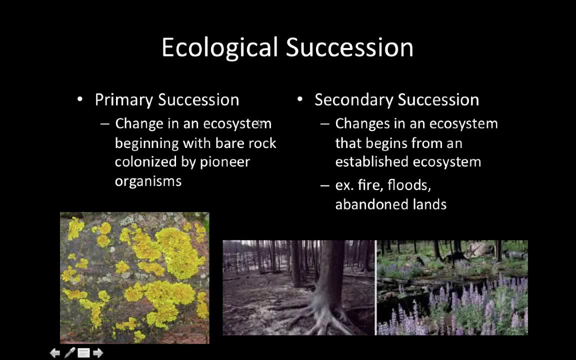 Those are two ways that we could do that. So that was how we estimate populations. Another way ecosystems change. besides their population growth is just their physical makeup. This ecosystems change through a number of ways, But we can break it down into two big categories: primary succession and secondary succession. 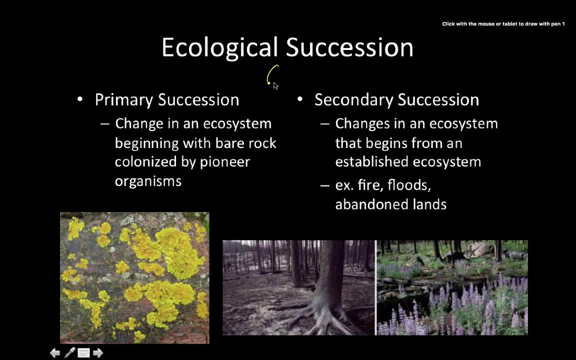 Succession really is. just when you think about succession, just think about it's a change over time. really, it's just aging, just aging. that's all it is. things are gonna look differently at the beginning than they do at the end. everything ages in one way or another. primary succession: the key takeaway is: 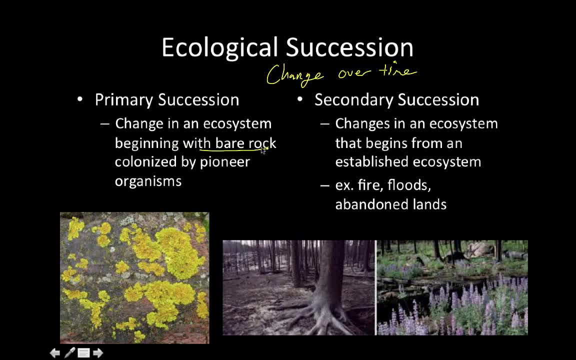 that this is a process that's beginning with bare rock and an ecosystem. there's nothing there but bare rock. it needs to be colonized by pioneer organisms, things like lichens, mosses, weeds, things that can grow in really tough environments. they can start the process of building an ecosystem from nothing. all right, so. 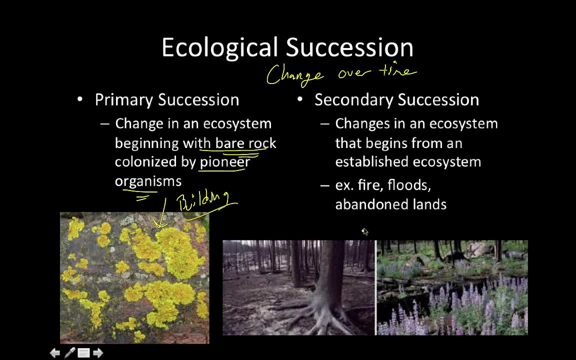 that's what we're doing here. they're building secondary succession is a start over an ecosystem, but it's really different because it's starting over from soil that's already there. so it's it's an established ecosystem that's just kind of been recycled. there's gonna be soil, all right. that's the takeaway here. there's rock here. 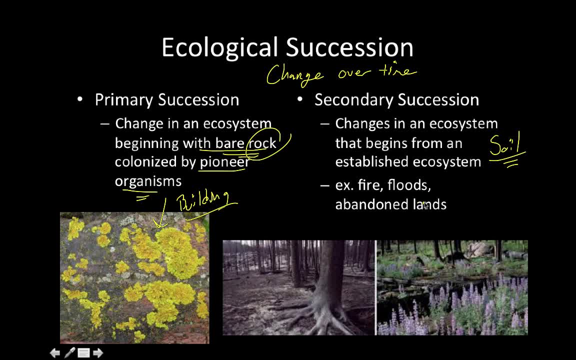 there's soil. what does this look like? well, maybe after a forest fire, everything's burned up, there's nothing living there anymore, but there's still soil. the ecosystem was established, there's stuff there, and then it's going to build from there. so this is a little bit faster because it doesn't have to. 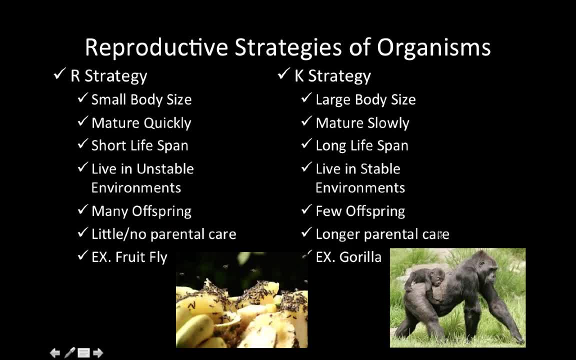 build that base. so organisms are going to grow from a fossil based ecosystem. So organisms, changing Organisms- have two characteristics, or two kind of lifestyles or reproductive strategies. we'll call them An R strategist and K strategist. A simple T chart in your notes would be awesome for this. What you go ahead and do is one of those. Boom, That's all you got to do. 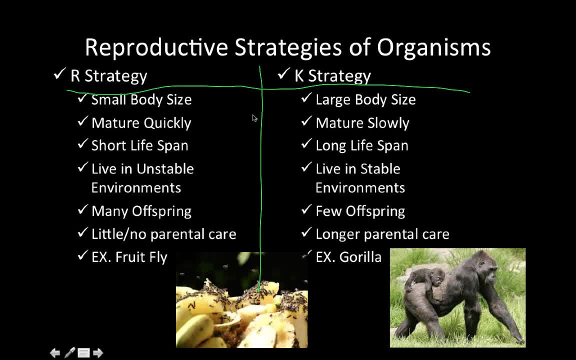 So what we're talking about here is really pretty simple, because everything on this side is the opposite of this side. But what is an R strategist? R strategists are things like: think about insects and how they live. They have small body size and mature quickly. They have a short lifespan. They live in unstable environments. They can have a lot of offspring, lay a lot of eggs. A lot of them hatch all at once. There's little or no parental care. There's no good mama fruit flies out there. They just let their eggs hatch and go about their business. 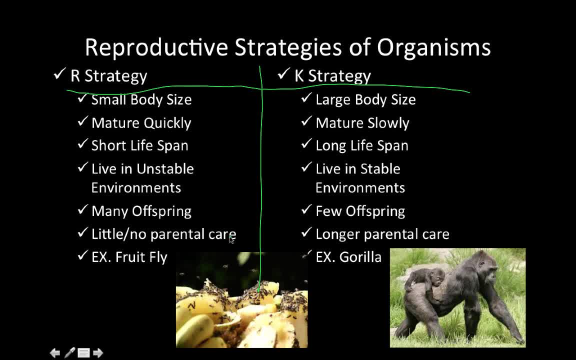 Right, That's one way to be successful. A lot of these organisms die early in their life, But some survive with little or no parental care, And it happens in a very fast rate. The other way to look at this is the K strategist. The K strategist has a large body size. It's going to mature slowly, have a long lifespan, live in very stable environments, has few offspring and longer parental care. 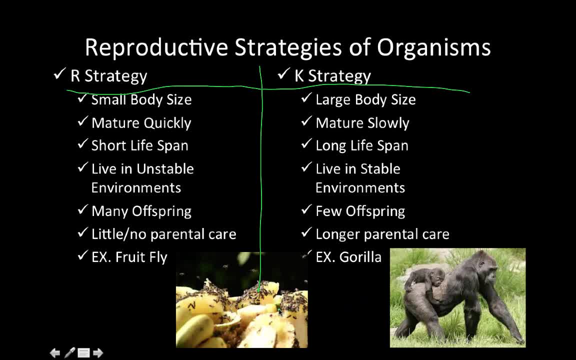 So you can see our fruit. Some flies over here have one way to go about surviving and reproducing, And over here we have a totally different way, And usually larger mammals end up like this, like elephants. humans and primates are going to fit into this category. 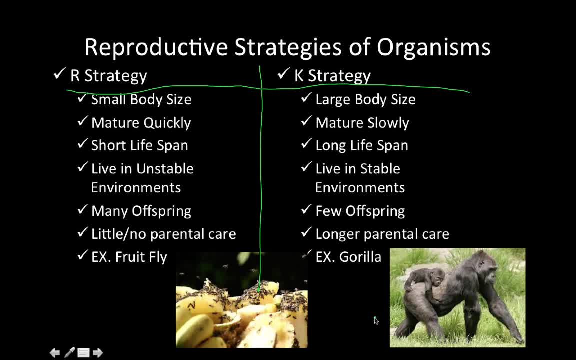 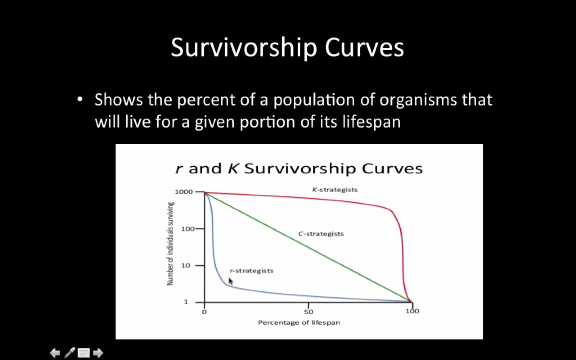 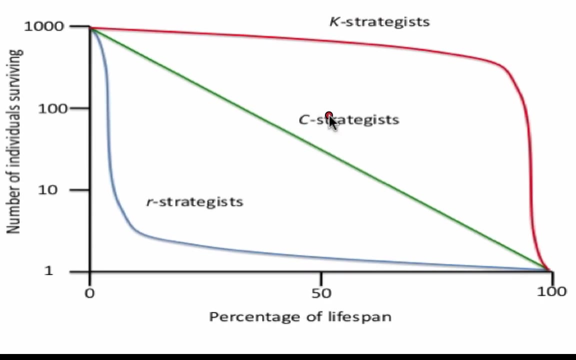 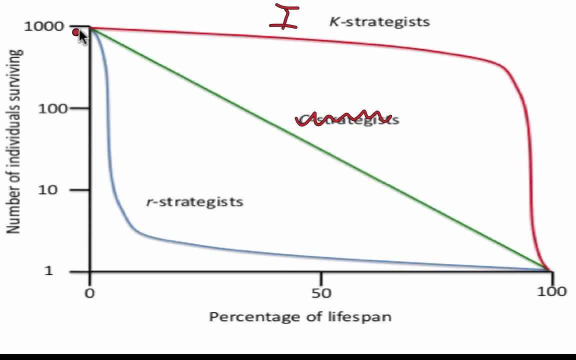 when individuals are surviving for most of their lifespan. so it's the survival rate over a percentage of lifespan. so if we're talking about our gorilla, it might have one offspring, but it's going to survive until almost a hundred percent of its lifespan, so it's gonna live to be an old adult. we have this type two. this: 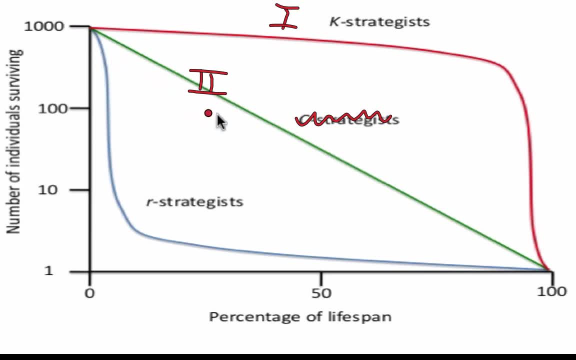 is again. this is kind of weird. this is a pretty constant death rate. so things like corals- and I don't like squirrels and stuff like that- there's some, just some kind of animals, that kind of fall in the middle that have a kind of a.